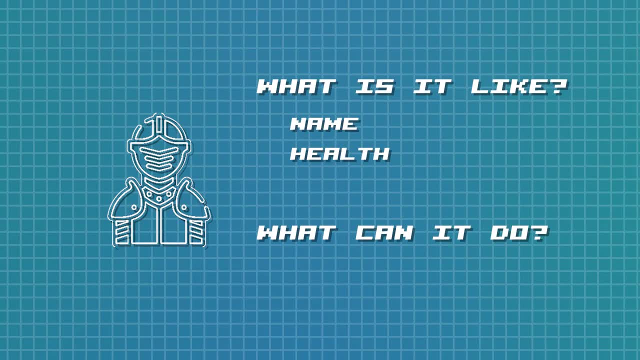 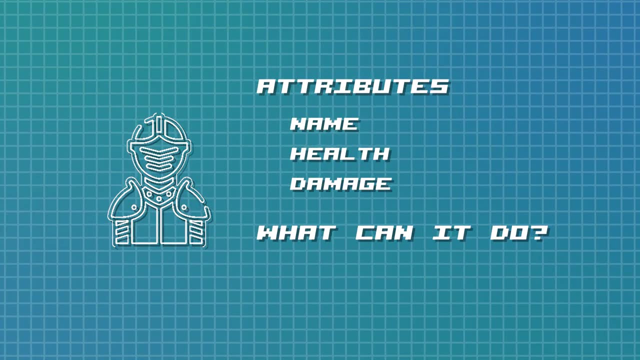 literally the simplest functional character. it should have a name, some health and image. These traits are what we call attributes of an object. To make a simple battle scene, we should also let this character attack. Every action we code into a class is called a method. 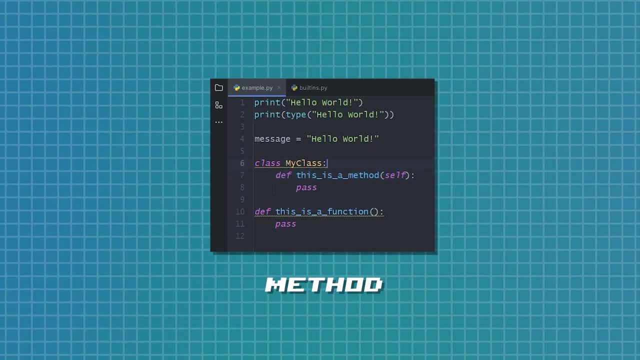 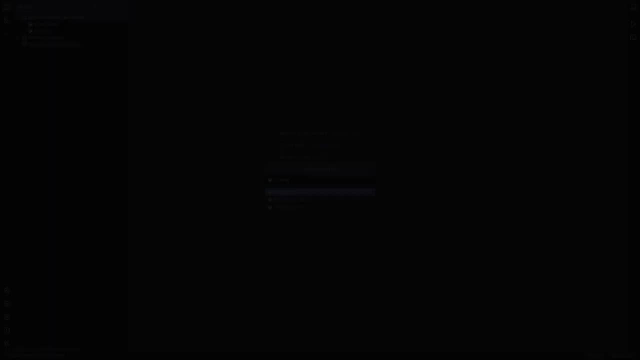 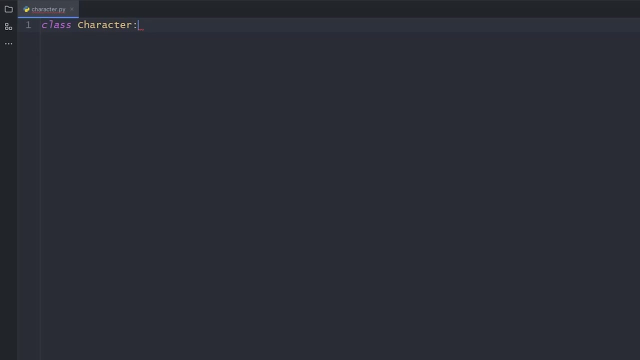 A method looks just like a function, with the difference that it's linked to a class. Now let's create the character blueprint and two character objects to simulate a battle. Let's start with an empty file. I call it characterpy. We define a character class this way. For classes, the naming convention is CamelCase. 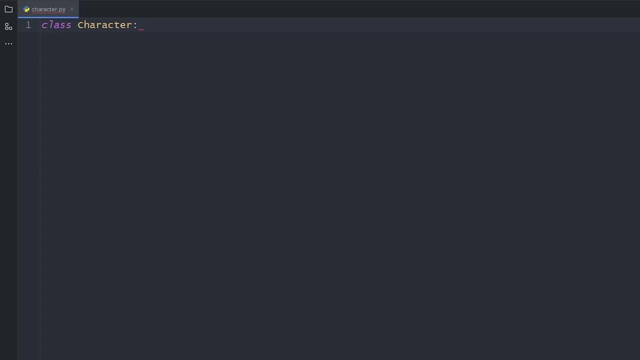 so all starting letters are capitalized. Then we define the special initializing method of this class. This is a double underscore method. They also call it dunder method or magic method. You will only come across this kind of methods if you create your own classes or look up Python's. 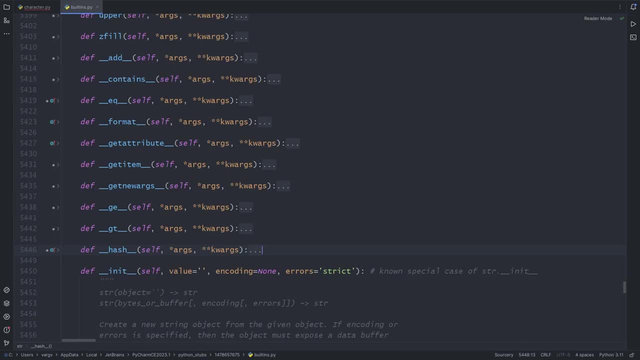 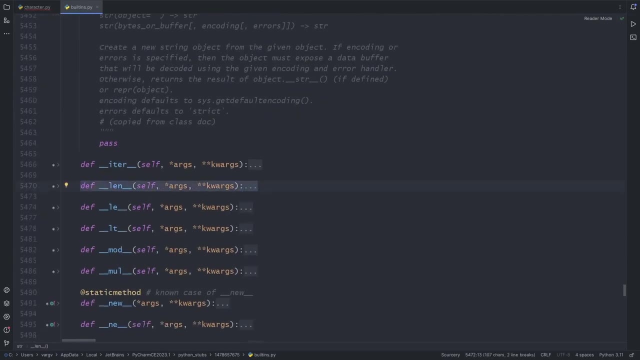 built-in classes. These are the ones that you shouldn't really overwrite. You could, but you overwrite default functionality with this Fun fact, built-in methods like len or other stuff you probably use so far are defined this way as well. So this init method is the one that 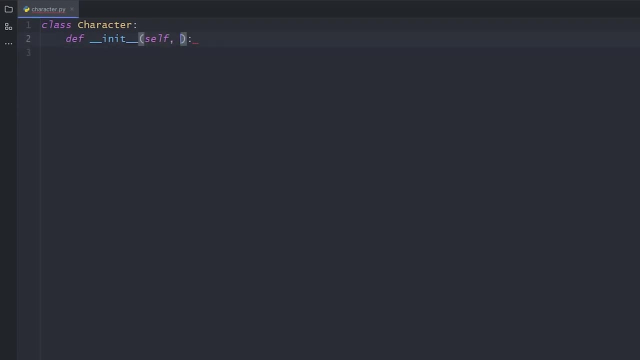 automatically gets called every time when you create a new object, so we can write the ones I mentioned: Name, health and image. We can even use type hints to remind ourselves what kind of data types we expect. The name is a string, while health and image are integers. 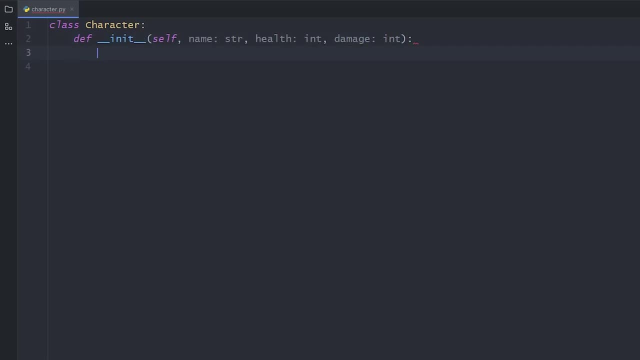 To store these input parameters in the object itself. we will save it right here in the init method To tell the code that we want to assign the values to the object. we can use the self keyword. You can name it anything. self is just a convention. So whatever name health. 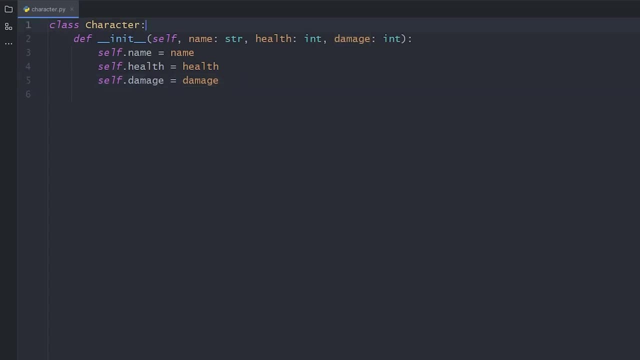 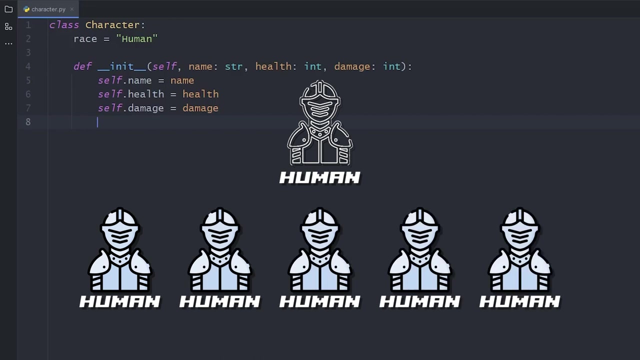 image you pass into this blueprint, the constructed object will hold these values. If you set variables before the init method, they will be shared across all instances of a class, So we can call these ones class-level variables. The ones in the init are unique to the created. 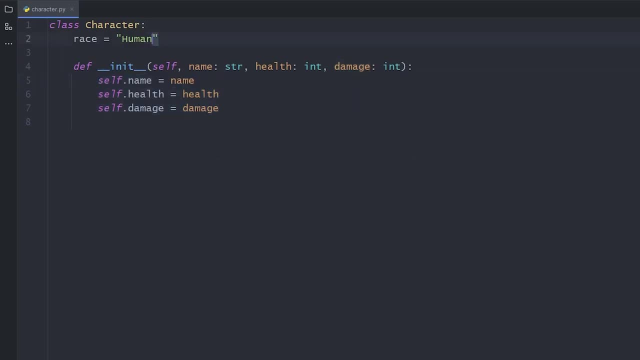 object. so these are object-level variables. Also, don't forget to set a maxHP property for the character. Alright, so the attributes are done. Let's define the attack method. It will accept only one input. that will be the target that we want to deal damage to. 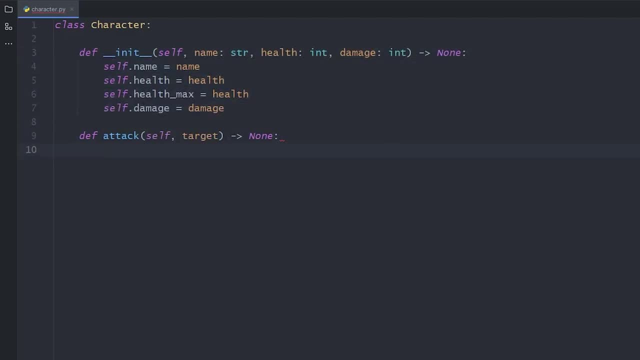 Since we will pass another character here that has the same fields, we can write: target dot. hp minus equals self dot damage. So the health attribute of the target will be reduced by the damage of the attacker. And to avoid going below zero we can use the max function. Easy as that. 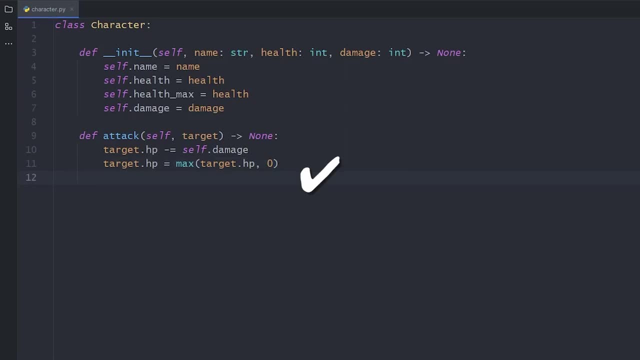 Good news: Our blueprint is completed. We can even create a battle scene. now, To keep the project modularized and the module files clean, I'll create a mainpy file that will be the entry point of the project. Now to create the characters, we have to import the blueprint from the characterpy. 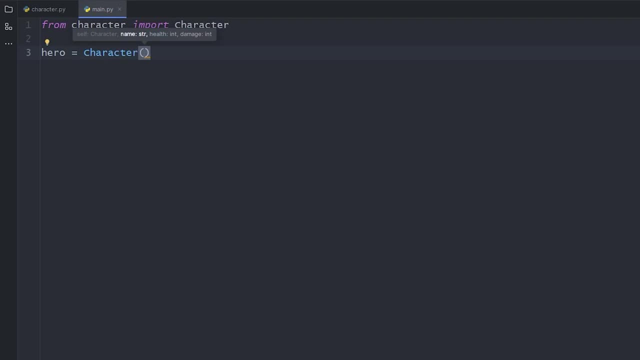 Let's make a hero object first, by calling the character class. with parentheses We can pass the required values either as positional or keyword arguments. I usually go with keyword arguments. this way I'm always sure what I assigned to it. Similarly, the enemy. 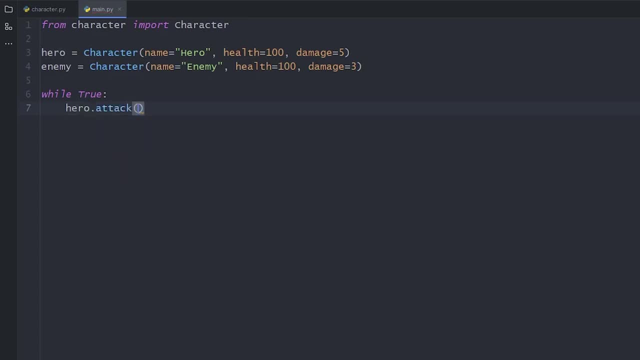 In our game loop we can start calling the attack methods of both the hero and the enemy. The hero will attack the enemy and the enemy will attack the hero. To see something, let's print their health to the console. To access the attributes of the created instances, we can type hero dot- any attribute you assigned. 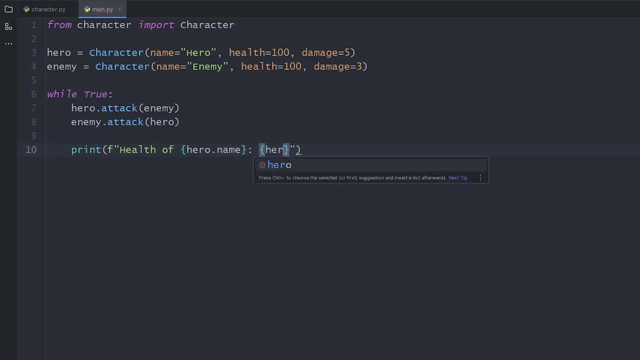 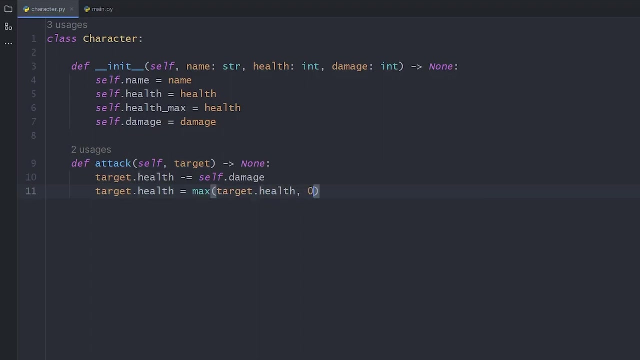 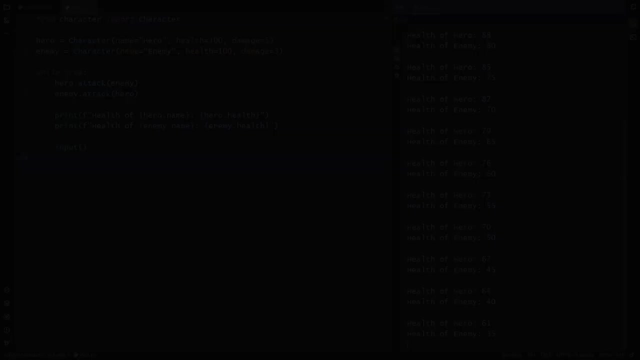 If you use a code editor, it should give you the recommendations automatically. Cool, And to control the flow of the code, let's include an input. Alright, It works. Now comes something pretty useful: Now that we have characters, we can give them weapons. Objects can hold other objects as well. 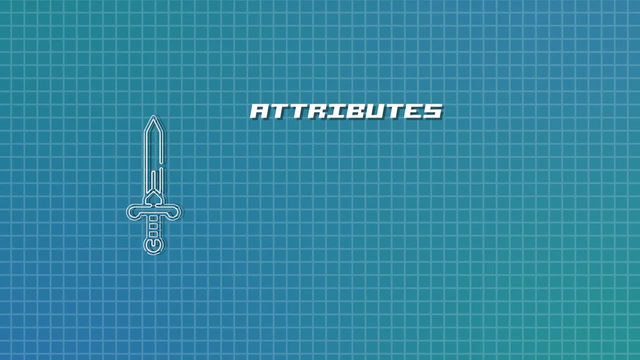 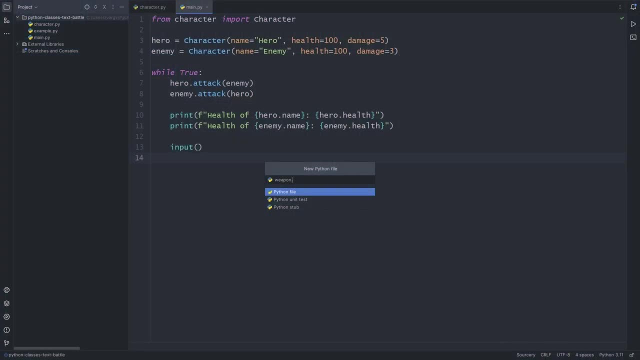 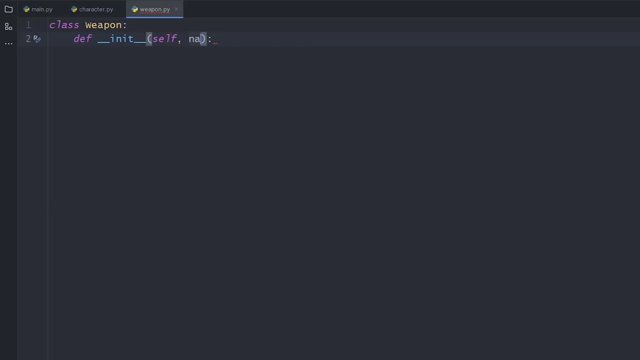 Think about it for a second. What properties should these weapons have? I'll go with name, type, the image and value, And that's it. Let's open an empty file. I name it weapon dot py. We can define a weapon class and in the init method we can pass the attributes I just mentioned. 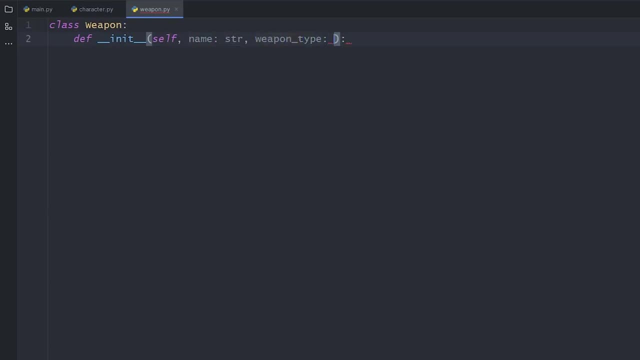 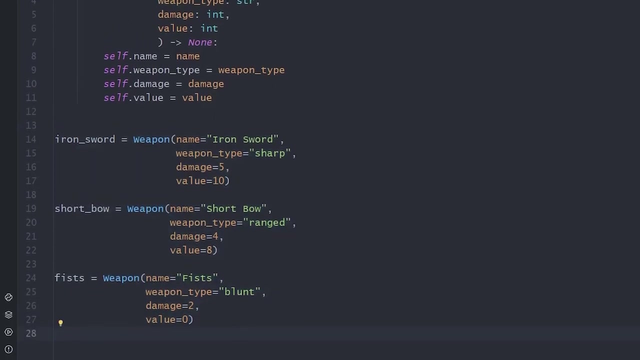 Now let's make 3 weapons: an iron sword, a short bow and fists. Now we have 3 objects that the characters can use. Now let's head back to the characterpy and type from weapon: import fists. 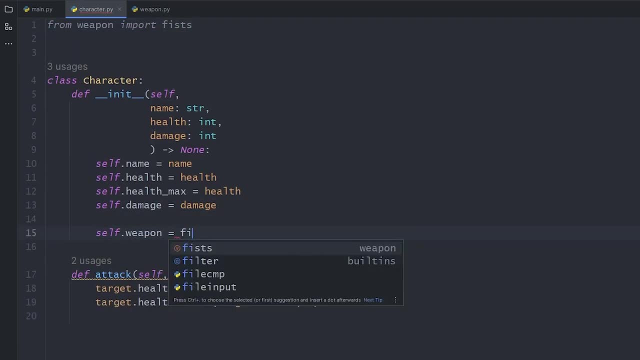 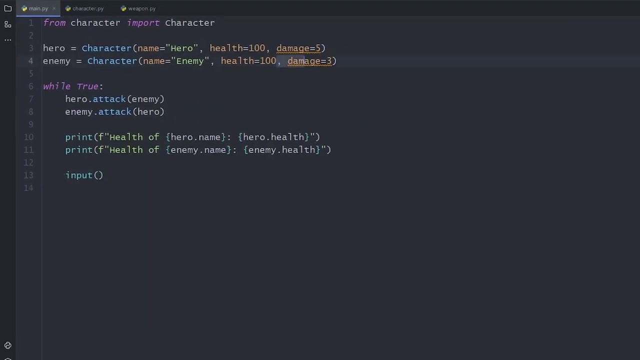 Then in the init method we can say: subweapon equals fists. All character objects will have fists as weapon. this way, Let's change the attack method now, and instead of our own dimmage we can withdraw the dimmage of our weapon. We can even remove the dimmage attribute of the character. 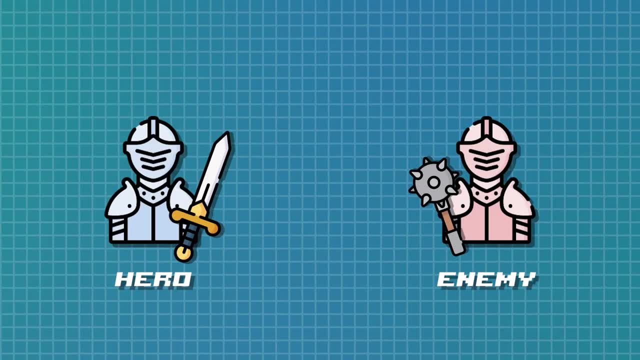 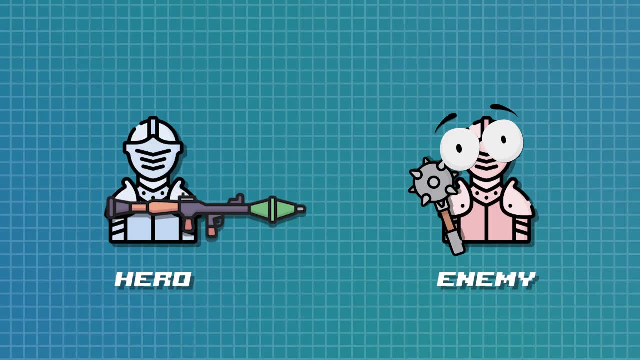 It's all coming together, Although I want the hero and the enemies to work differently. The hero should be able to change its weapon by equipping or dropping one. One enemy should have the same weapon all the time, and I want to control this when creating. 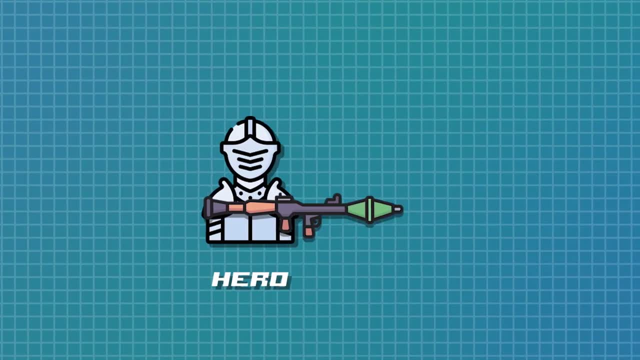 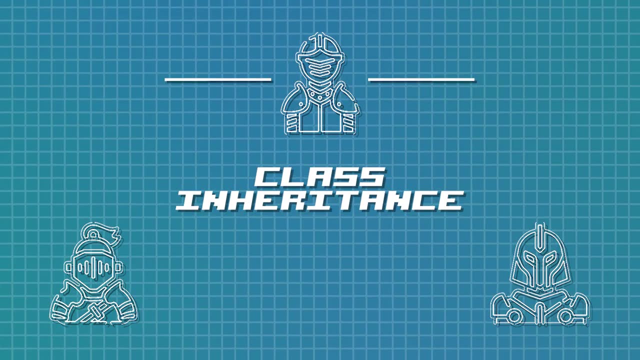 this specific enemy. So I want the hero and the enemies to function differently. And with this we reach the topic of class inheritance. Now that I have a complete class, I can create as many subclasses out of it as I want To do. that let's type class hero. 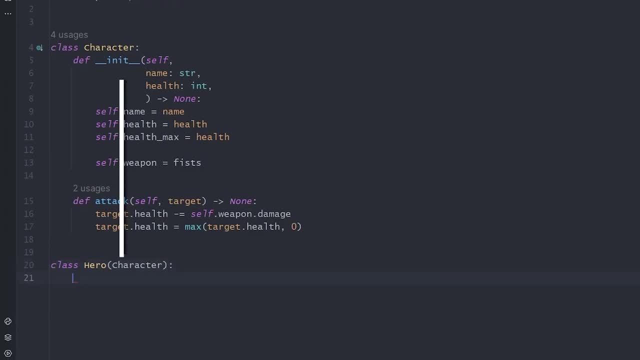 And put character in parentheses. This way we're referring to the parent class. This means that the hero subclass will inherit all the stuff that we created in the character class, But, just like before, we need to initialize the hero object that we create with this blueprint. 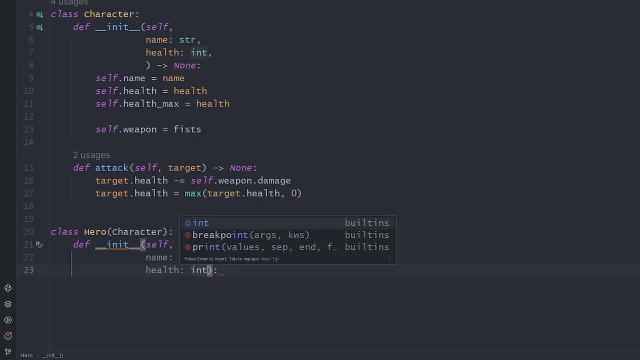 Again, our hero will have a name and some health. But, unlike before, I won't save these variables here. Instead I pass these arguments to the parent. init To do that we can call super. That refers to the character. Then init: name and health. 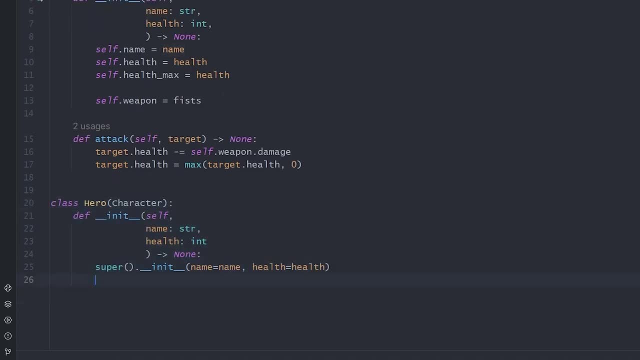 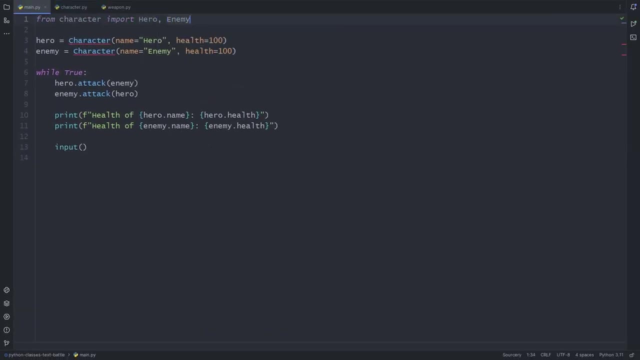 This way we initialize the core of our subclass. Let's duplicate this for the enemy subclass as well. And now, if we head back to our mainpy, we can import hero and enemy instead of character and call them with the same arguments. It works fine, just like before. 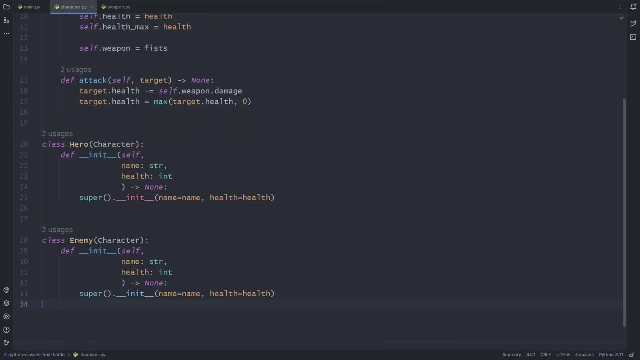 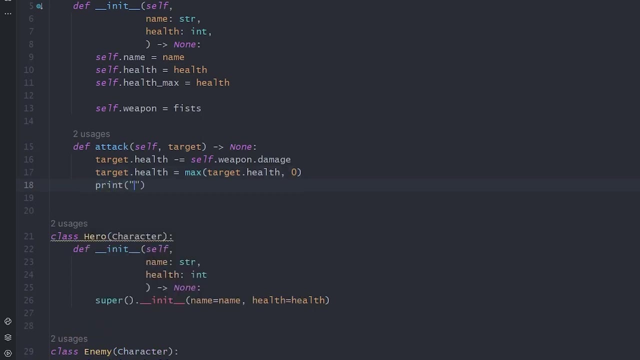 You can notice that we didn't define attack methods in these subclasses, but we can still call them. That's because they inherit it from the character parent class. And while we are here, let's print some stuff to the screen with an f-string. 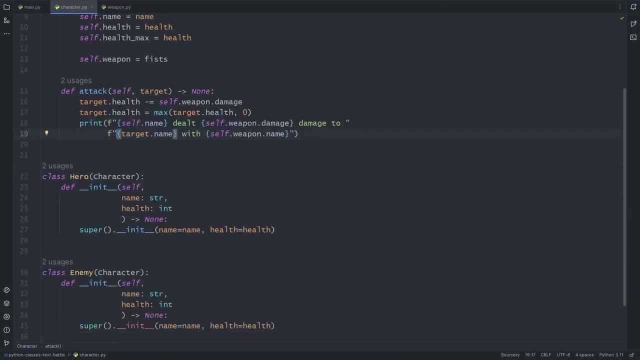 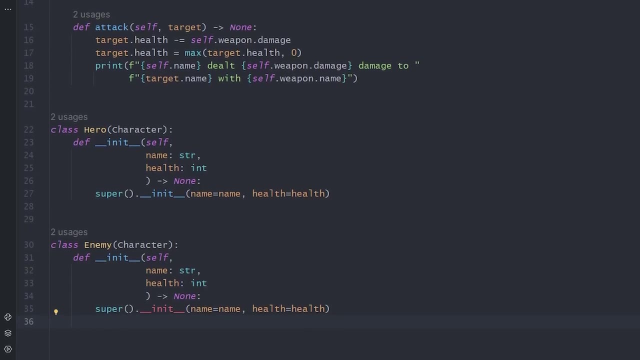 Now, if we try it, it looks even better. Now we can implement the weapon logic inside hero and enemy. Let's start with enemy. that's the easier one. Right now, all characters have fists For the enemies. I want to overwrite this right in the init method. 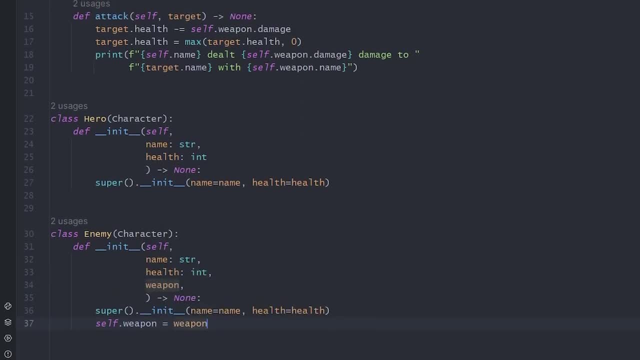 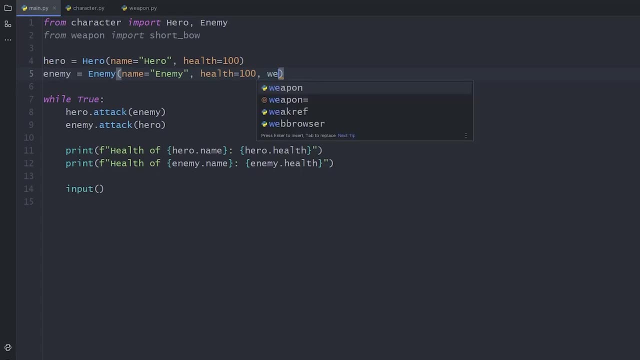 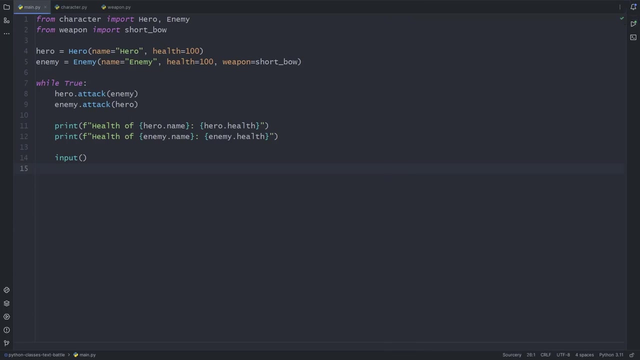 When I create one. So if we import another weapon into the mainpy, like bow, and pass it as the weapon argument of the enemy, it will use this bow instead of its fists. Great progress. Now let's see the hero. Instead of passing a weapon argument when creating the hero object I want to define. 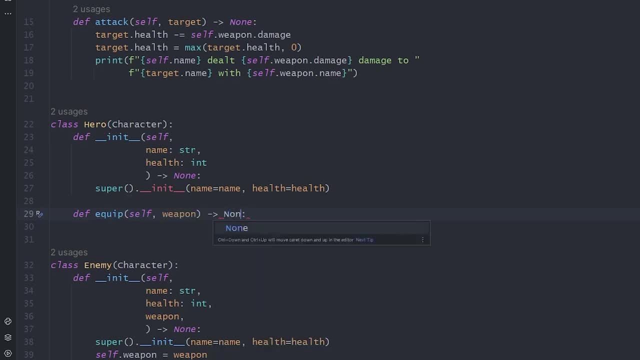 an equip method. We can pass the object here and this object will overwrite the current weapon of the hero. Yeah, It's the same as if we called heroweapon equals something outside the class, but we could extend this method if we wanted to. 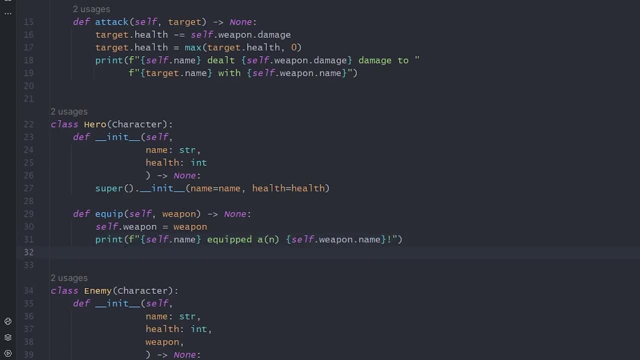 Like printout: you equipped a weapon, etc. Let's make the other method now. With this one, we simply set our weapon to the default one. To do that, we need to set a default weapon up in the init method first. 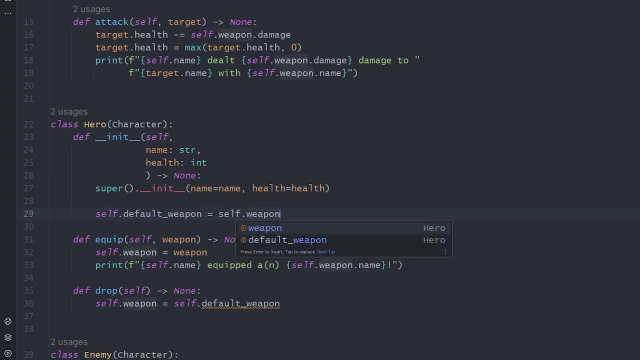 Remember, we have a selfweapon in the character init, so we can just type selfdefault. Defaultweapon equals selfweapon. Now our default weapon is the fists, so whenever we drop our current weapon, it will be reset to fists. Cool. 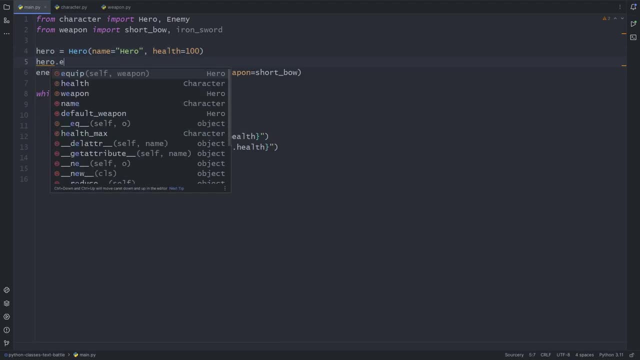 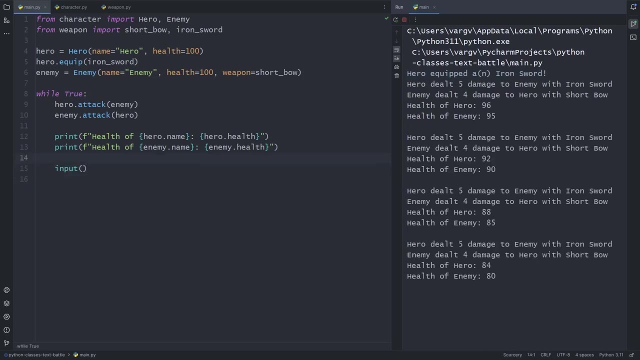 Let's import the iron sword to the mainpy and equip it for the hero. We can see it in action as well. If we drop the weapon, the hero uses its fists, Just like before. We can see it in action as well. 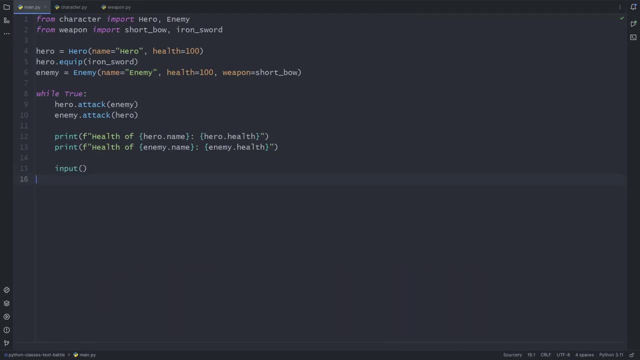 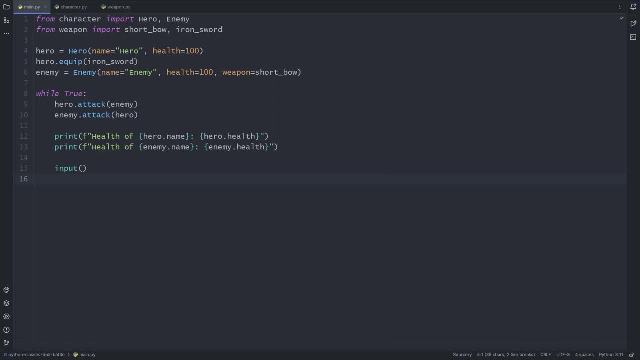 We can see it in action as well. We can see it in action as well, Just as we wanted. Now, only one thing is left for this video. This looks pretty ugly, so let's make proper health bars. In my last video I already covered the topic, although not with classes. 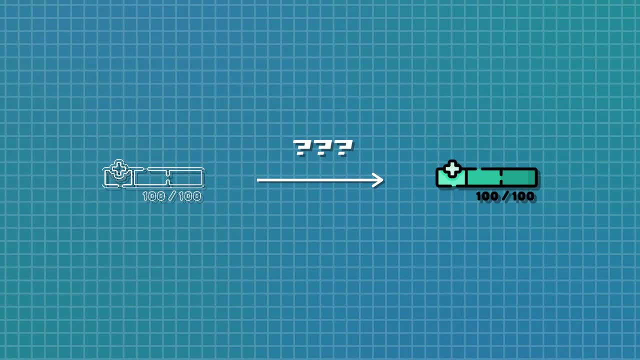 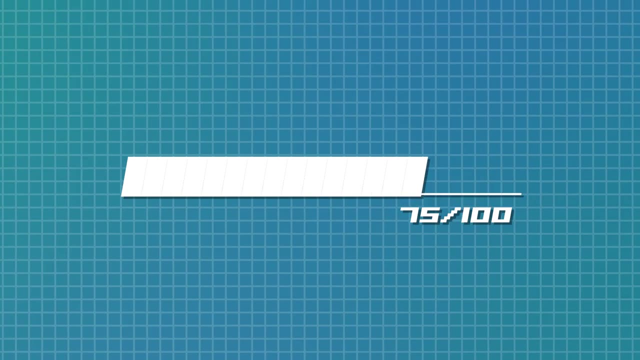 Let's think about health bars. with OOP in mind, A health bar should have the following properties: Length, maximum value, dynamic value symbol for both remaining and lost amount. its decorating barriers. if it's colored, its color, and that's it. 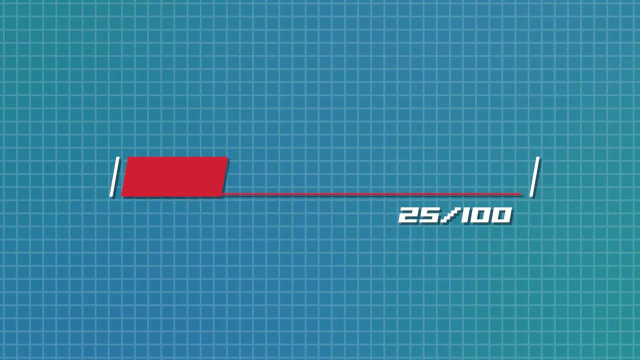 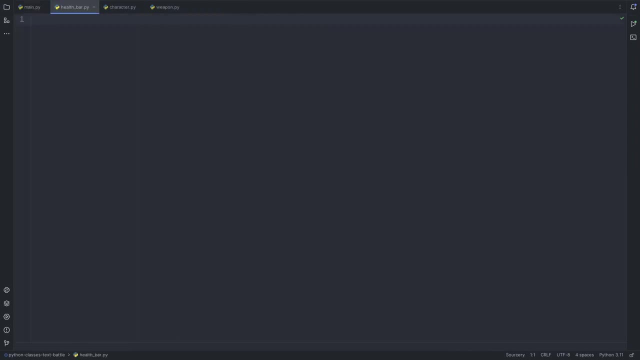 It will have two actions: An update method to update its current value and a draw method to print it to the screen. Let's get coding. I'll make a healthbarpy and right here, before I make the class, I'll import the built-in. 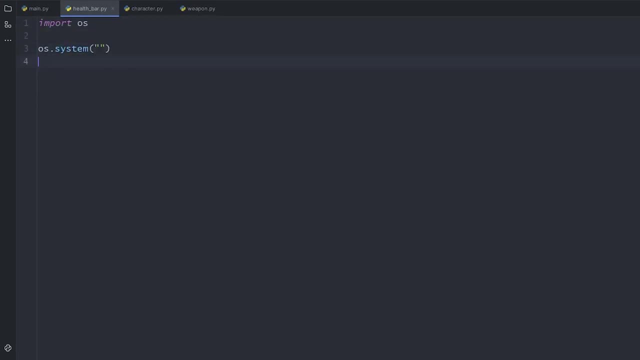 OS library. After that I call its system method with an empty command. This is a hotfix if your console doesn't print colors properly. Now we make a healthbar class and to the init method we can pass length max value. 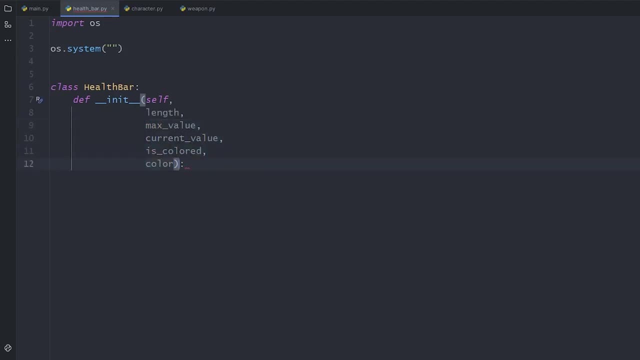 current value isColored and color. But since we're big brains, instead of max value and current value we can pass an entity object that will be a character and we can reach their health values directly. So let's save all these. 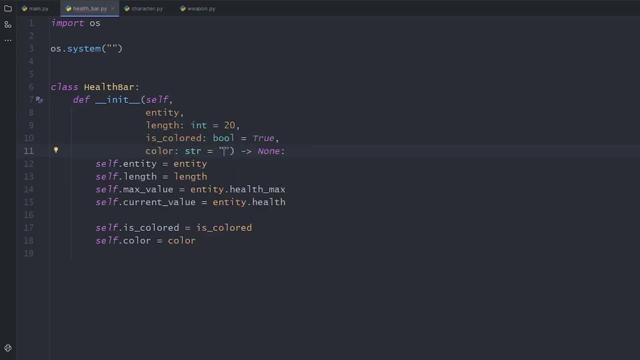 We can even give default values to these parameters. so if we don't give these arguments when creating the healthbar object, It will refer to the default values. But what about the other properties? I mentioned The symbols and the decorating barrier. I assume that these will be the same for all healthbars, so I define them on class level. 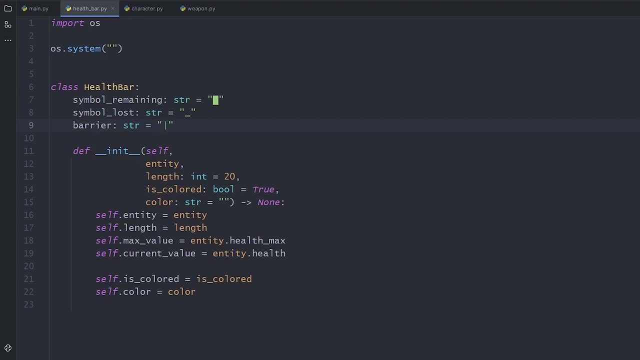 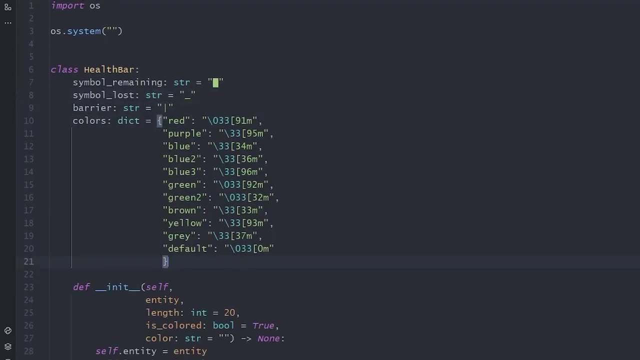 I could put length here as well, but what if I want longer healthbars for bosses, for example? Ok, now what about colors? I cannot just use a string for that, So I made a couple of color values here that I store in the colors dictionary. 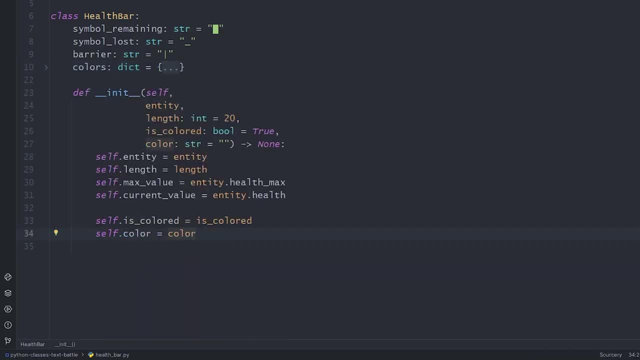 And in the init method The color property of the object will be accessed from its colors dictionary by the color parameter. We can write it all in one line. First we try to find the color key in our dictionary and its corresponding value. So if we pass blue as color and the colors have blue in it, the bar will be blue. 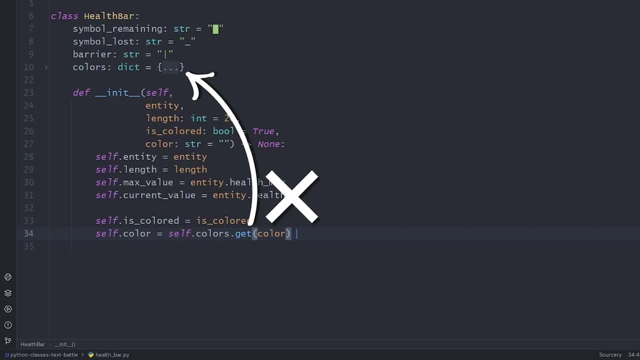 If the word is not in the keys, the statement will be false, And if it's false, we should set a fallback value. That should be the default. no color value. Ok, We can see for ourselves that color is bulletproof Cool. 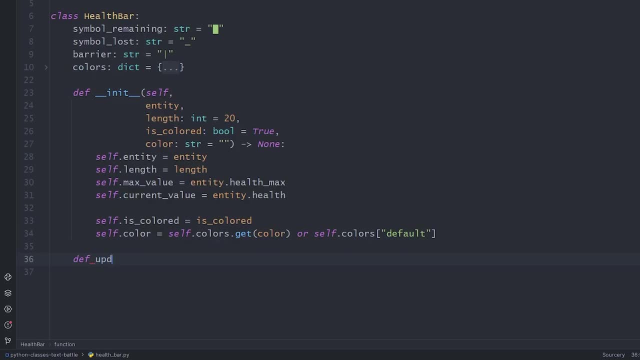 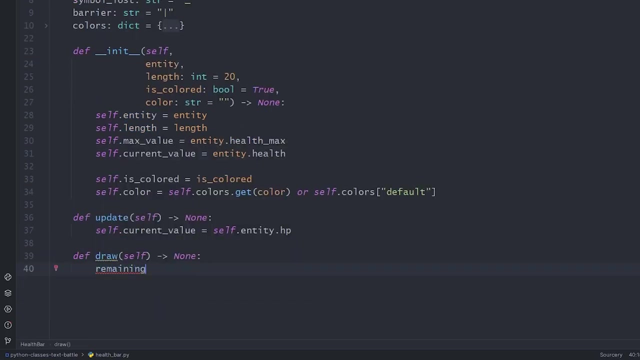 The init part is complete. Now only the two methods are left to make. The first one is the update method. We can set the current value of the healthbar to the health of its entity. The next one is the draw method. Here I want to print the health of the character as a healthbar, and with numbers. 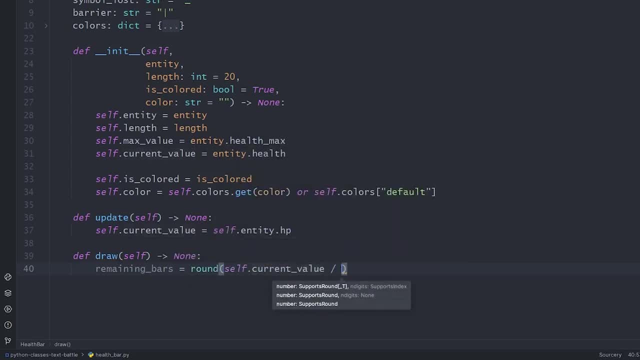 As before, the remaining bar amount will be the length multiplied by the ratio of the current and max values. Ok, To get the lost bars, we simply withdraw the previous value from the length. Now let's print the health with numbers. Then we can make a pretty long f-string. 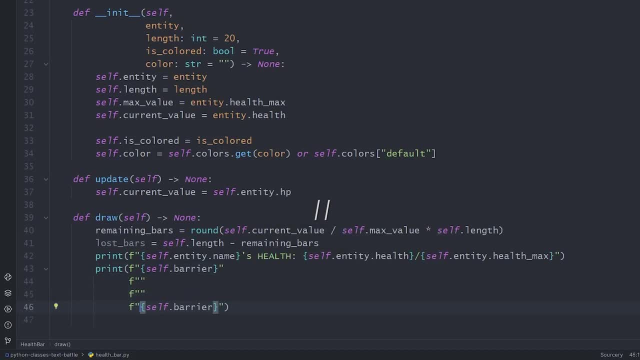 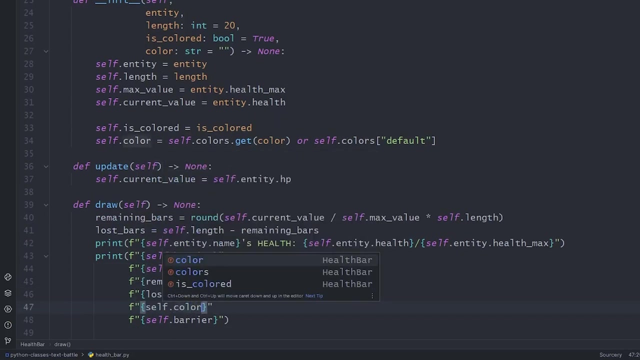 We put one barrier to the front and one to the back. Between them comes the remaining amount with its corresponding symbol, same for the lost amount. And don't forget to add the coloring part before and after these symbols. We start with the color attribute and end it with the default color. 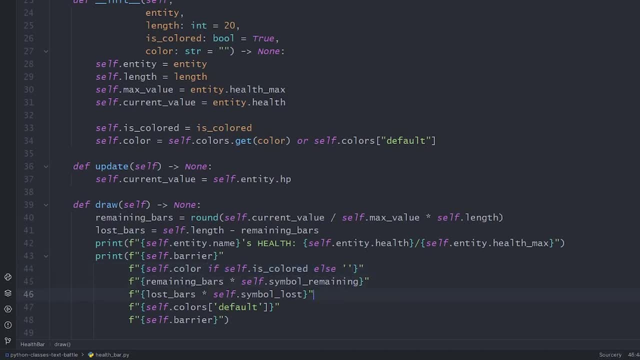 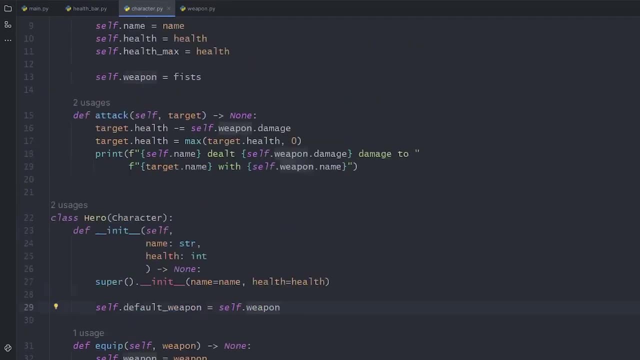 But only if the healthbar is colored. Let's use one-line conditionals here. Now the draw method is completed. Before we display these bars, let's add them to the characters. If we head to our characterpy, we can import this healthbar class. 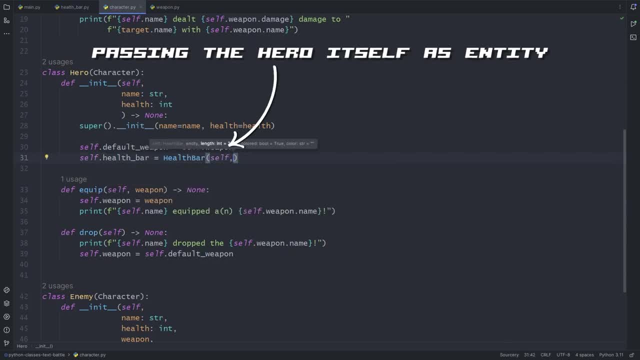 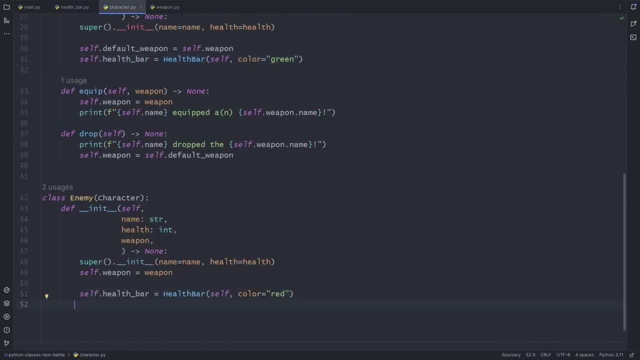 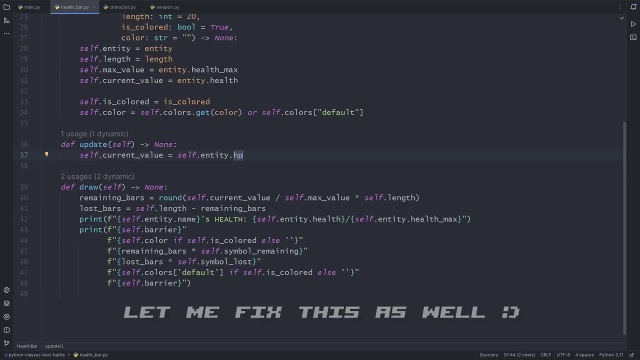 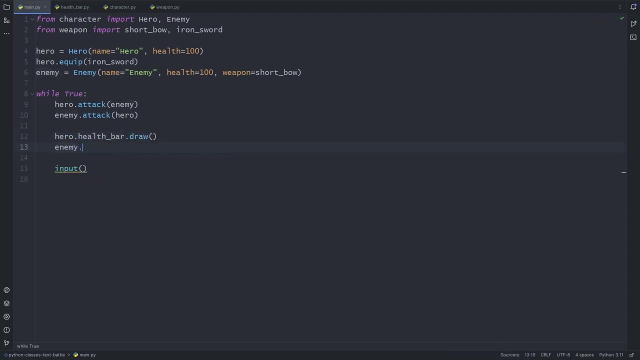 The hero will have a healthbar object And the enemy gets one with red color. We can also extend the attack method with the update method of the target's healthbar, so it will be refreshed right after the action. Now, if we go to our mainpy and update our game loop with the draw methods, we can see: 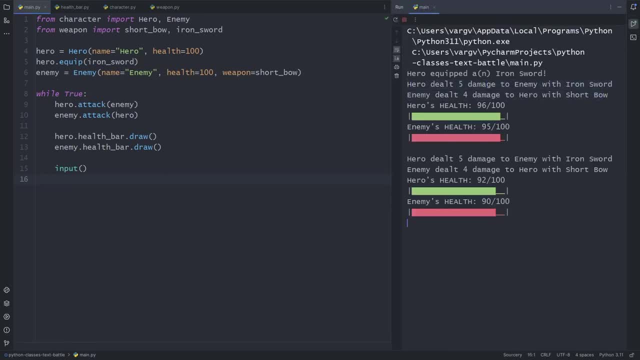 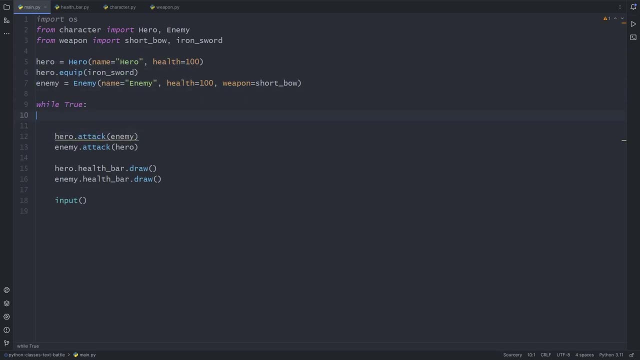 all of our hard work pay off with a very cool battle scene. Ok, If you'd like to clear the screen in your terminal, you can import os in the mainpy and call ossystem and put cls in parenthesis at the start of your loop. 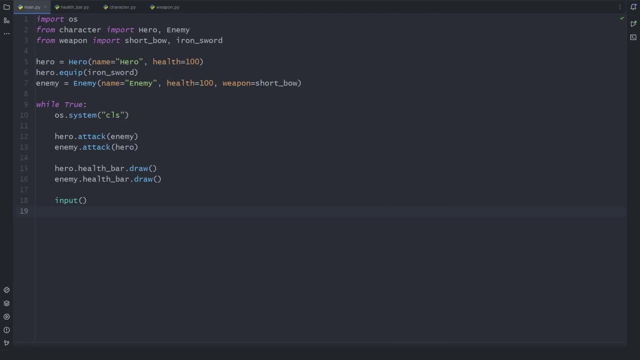 Now it looks even better. Alright, this was my comprehensive Python classes tutorial. I hope you enjoyed it and either learned some cool new stuff or had a refreshing experience. If you did, please leave a like and give me some feedback in the comments. 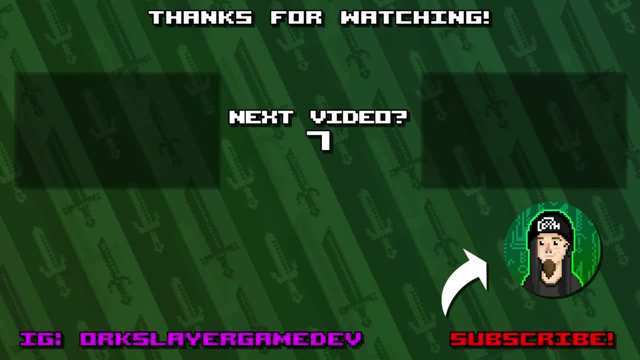 And, of course, subscribe for more. See you guys, Stay safe and take care. Bye. 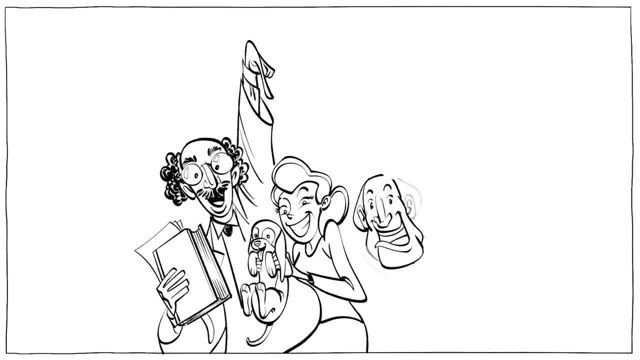 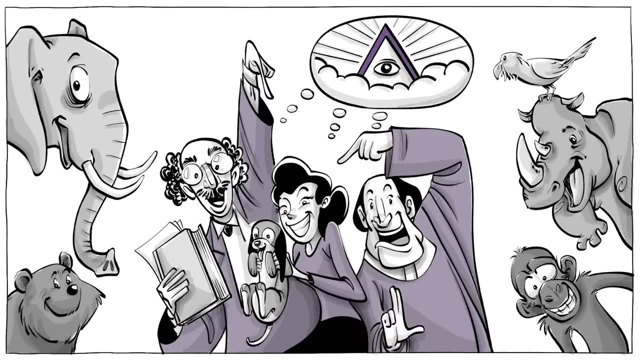 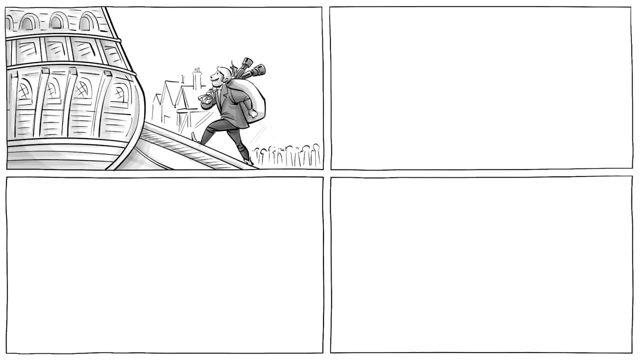 At the beginning of the 19th century, most people in the Western world had a solid theory about our origins: All creatures were formed by a single creator. But then, in 1831, a 22-year-old student decided to go on an expedition that would change everything. The young man spent years on remote 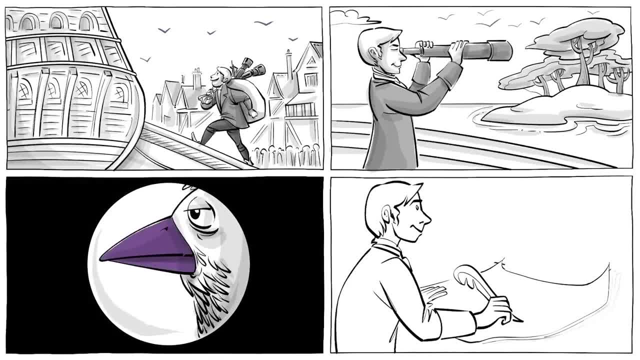 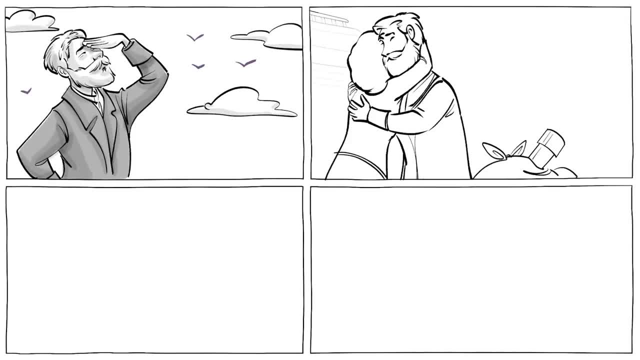 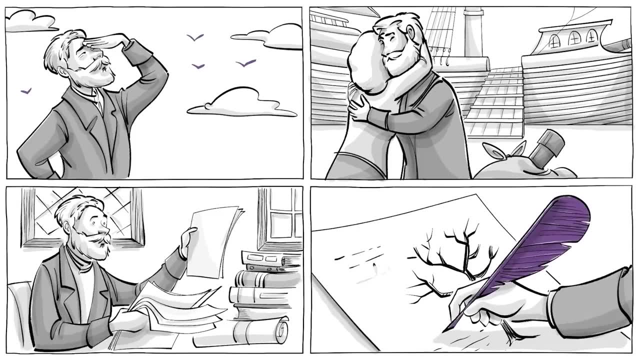 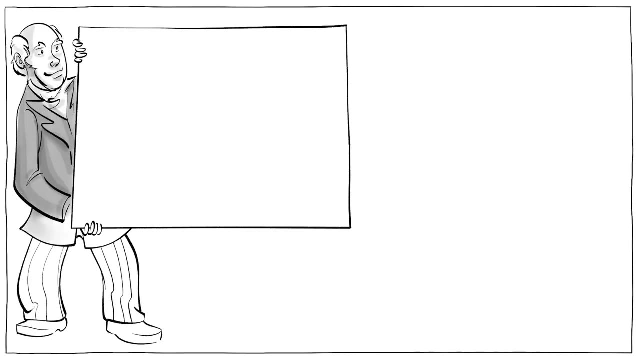 islands, investigating living organisms and taking careful notes on their differences. After close to five long years, the man returned home. He organized his findings and started to write his own theory on the origin of species. Decades later, in 1859, Charles Darwin, supported by the work of Alfred Wallace, 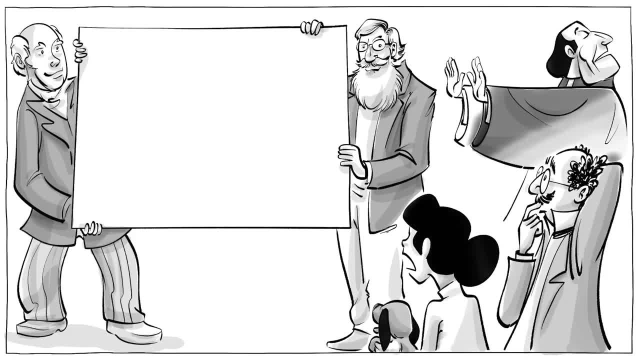 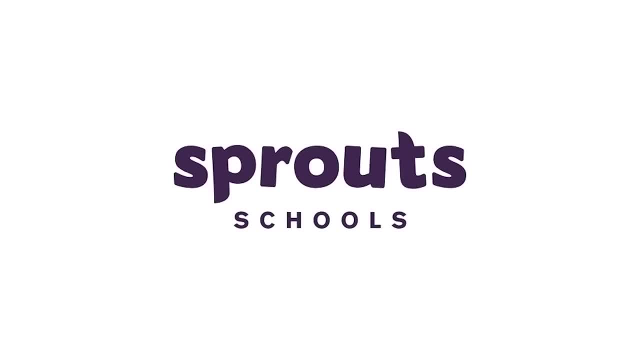 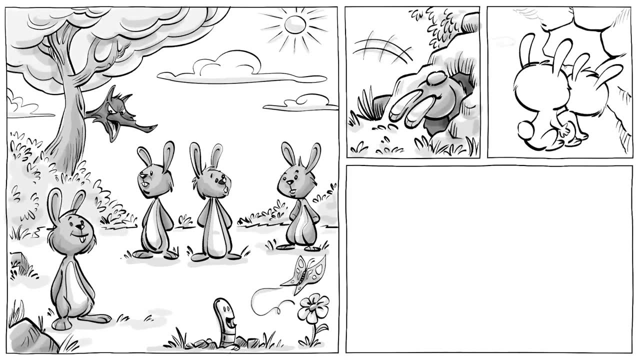 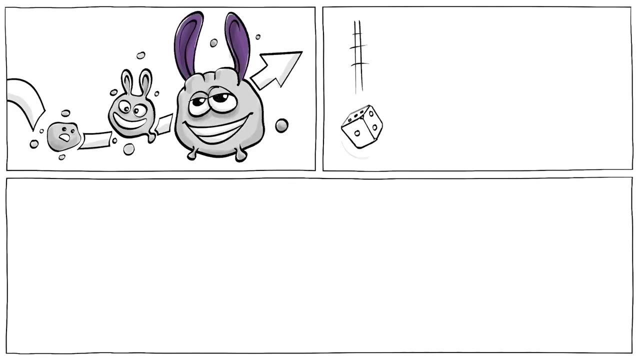 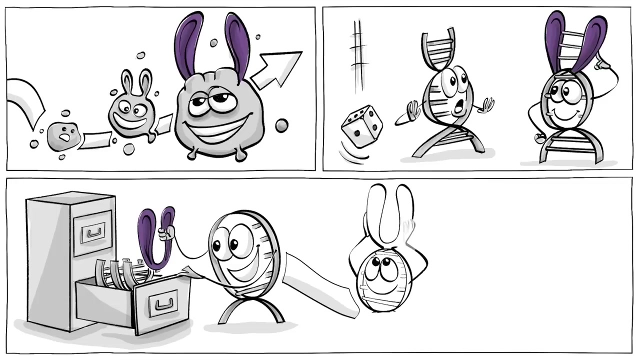 challenged the status quo with his theory of evolution based on natural selection. Natural selection is the process through which populations of living organisms adapt, reproduce and change. This is possible because organisms evolve when random mutations happen in the DNA of reproductive cells Stored in cells. the DNA contains instructions that 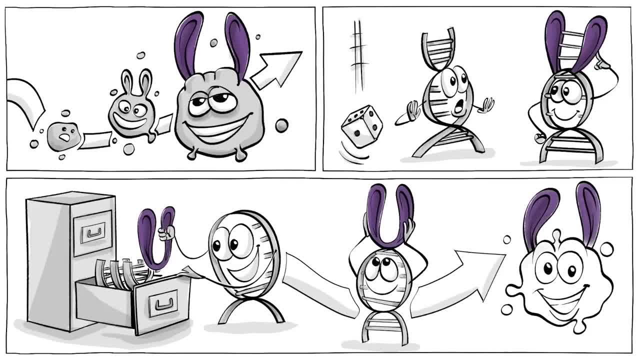 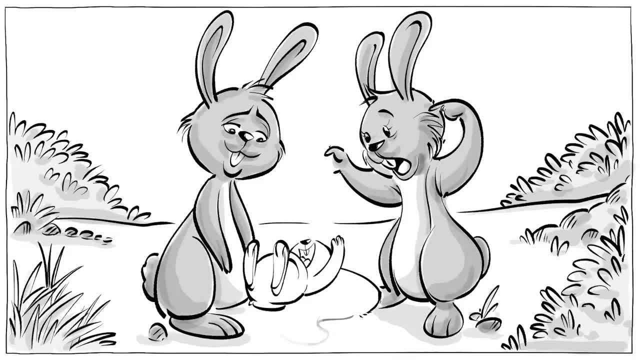 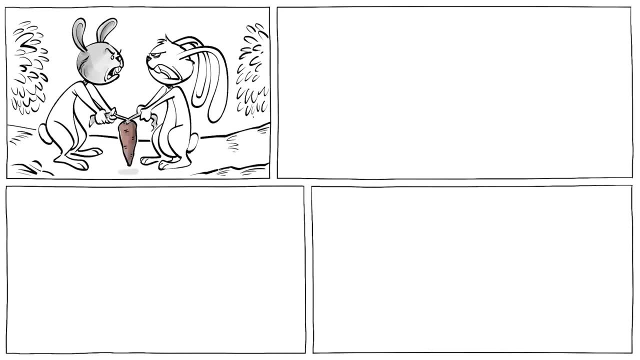 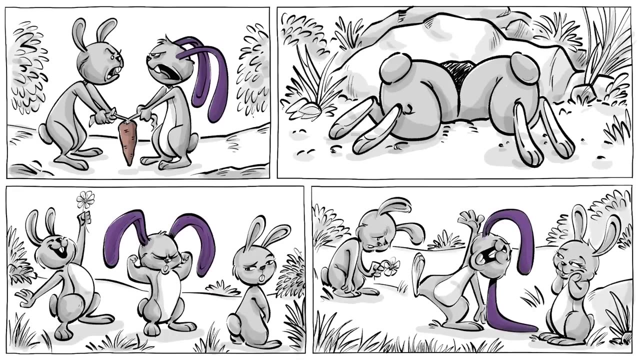 determine an organism's characteristics early after conception. For instance, two animals with a particular features can have a baby with very special ones. Since most of us are in competition for limited resources, territory or potential partners, certain traits are beneficial while others are not.